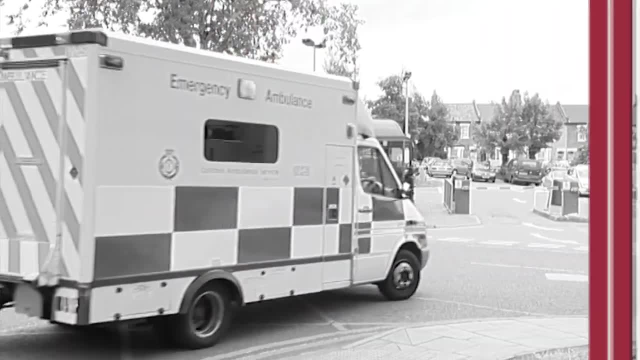 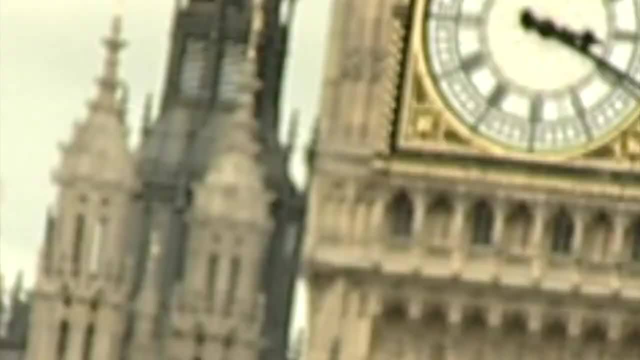 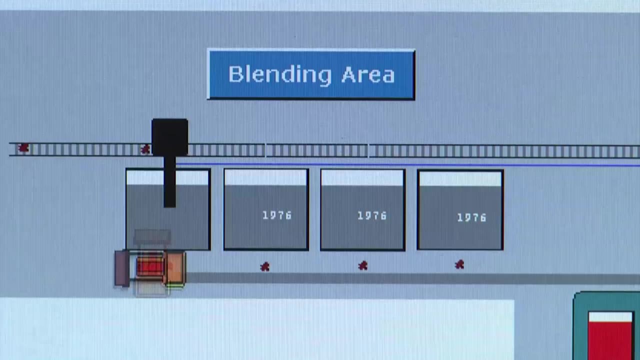 our weekly groceries. It helps save lives. It drives business and government, Without OR, the modern world we take for granted wouldn't exist. There has never been a better world for us all. Thank you. better time to be an operational researcher? Today, most organisations have masses of data. 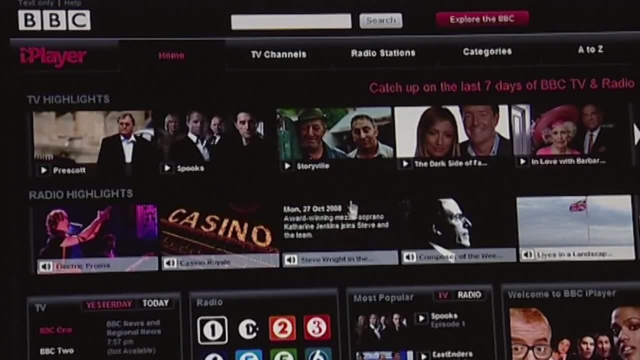 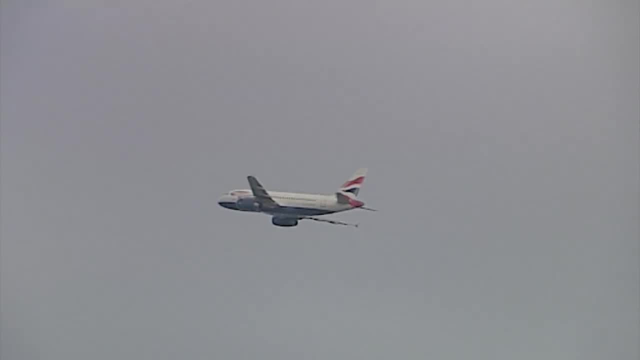 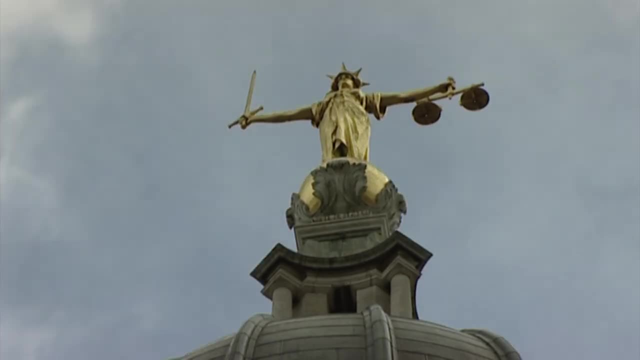 The ways we communicate are fast, computers are sophisticated and powerful, And the business world is now investing heavily in putting operational research at the centre of what they do. This is not maths in theory, but maths in the real world, making a real difference. 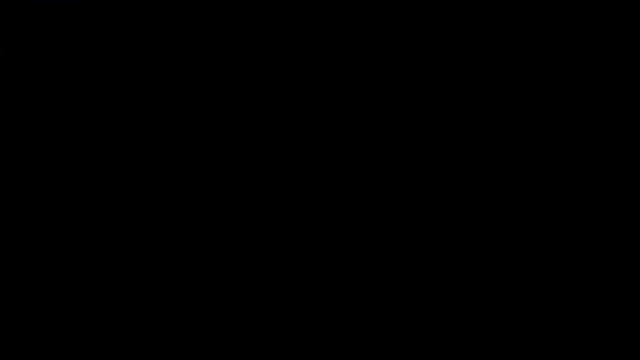 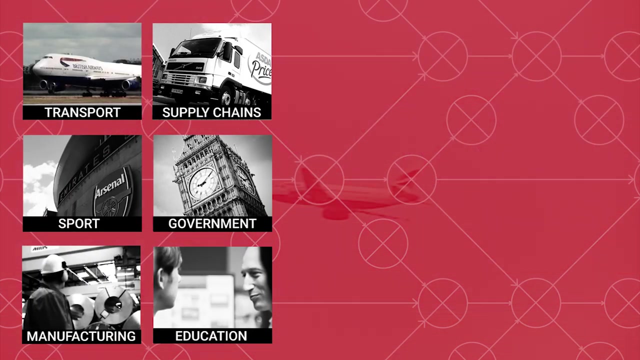 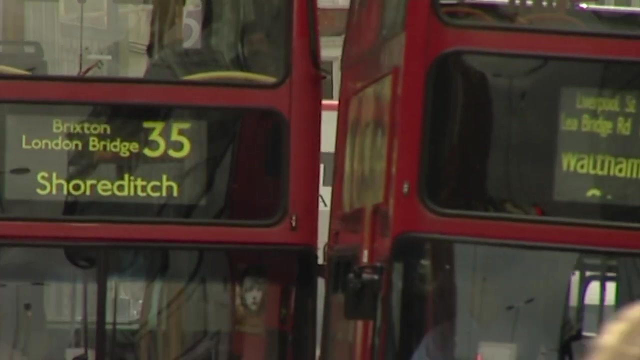 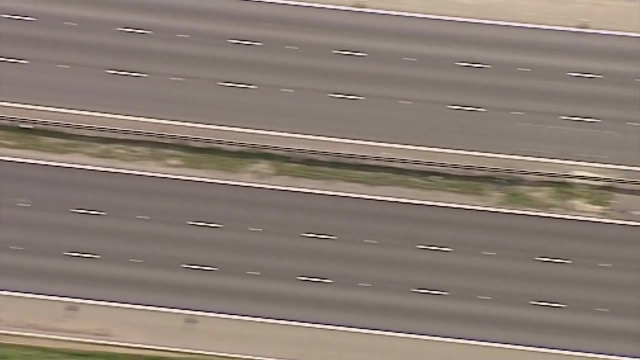 Never before have so many people or products needed to be moved around the world. As passengers and consumers, we expect everything to run smoothly, Whether we are buying flights, commuting to work or wanting food readily available at the supermarket. For business people, it is important to know what they are buying and what they are selling. 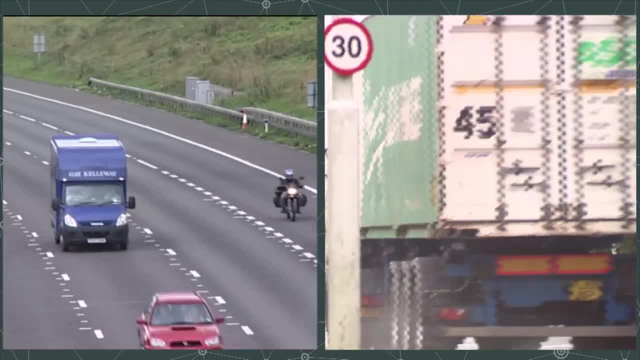 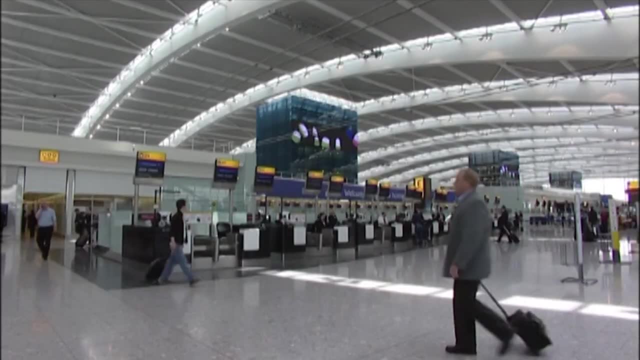 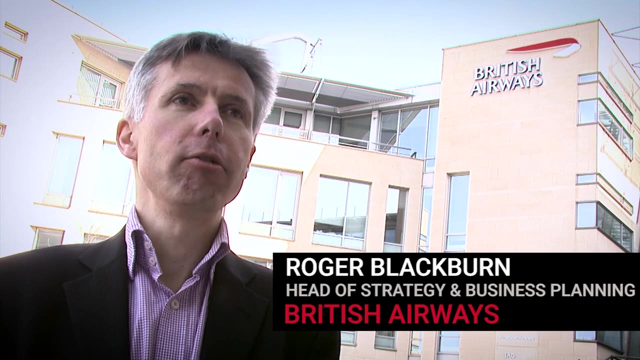 For businesses, moving people and products around can be a complicated and expensive matter. Here at British Airways, getting the maths right can make passengers more satisfied with the service and make millions of pounds worth of difference to the business. The OR department of British Airways has been here a long time. We influence a whole range. 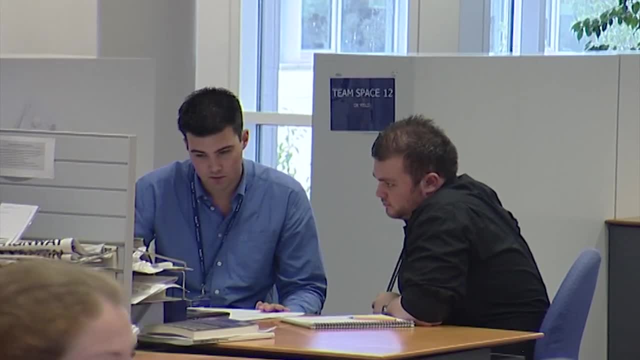 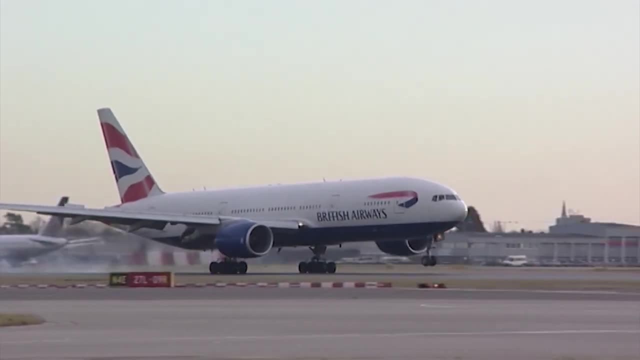 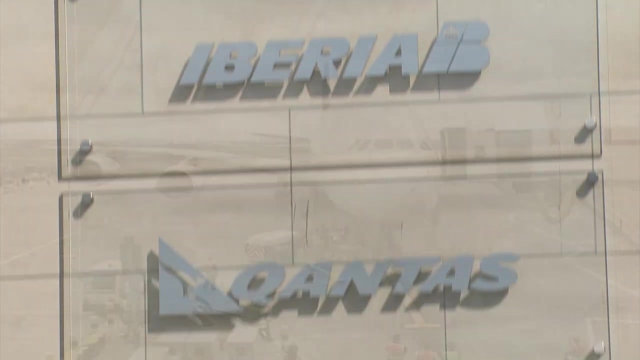 of decisions. We are a big, complicated business and OR thinking is pretty critical to taking the right decisions OR helps influence a range of decisions. We make decisions across the business right from which aircraft should we buy, where we should fly, who our alliance partners should be, how we should board the new A380s, how. 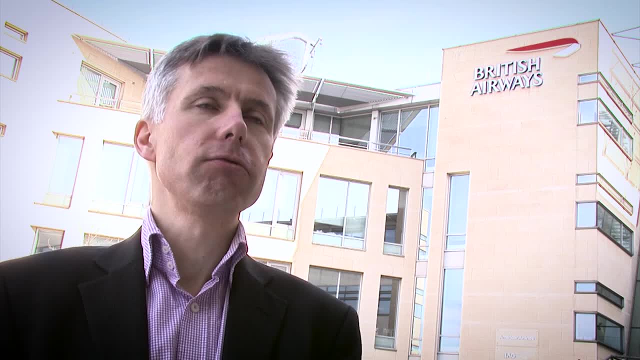 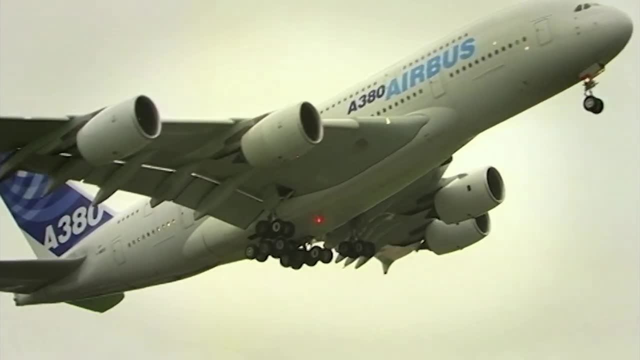 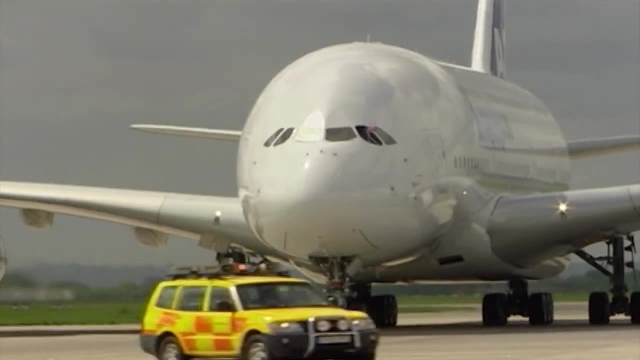 many tickets we should sell, of what type, what our customer data is telling us right across the range of the business. This is the Airbus A380, the largest passenger aircraft in the world. These new aircraft are a fantastic opportunity for British Airways to expand. 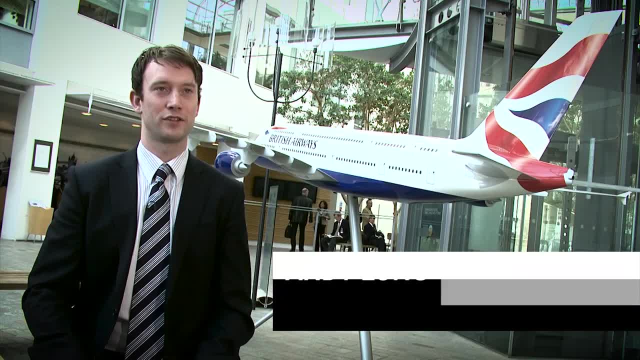 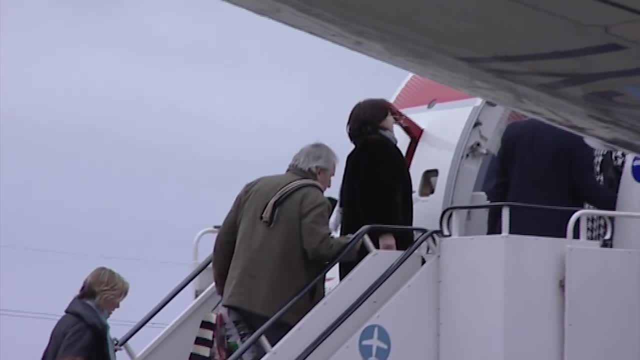 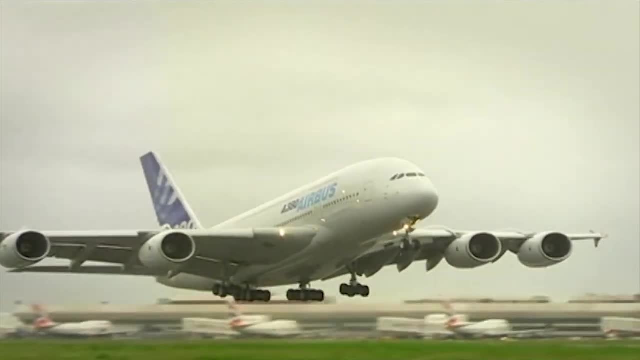 Without this opportunity comes risk. We've never operated an aircraft this big before, and getting it wrong can have huge impacts on the entire operation. There could be delays, which would impact customer satisfaction, and getting it wrong could incur additional costs, which obviously will impact profitability. The business was interested in seeing how. 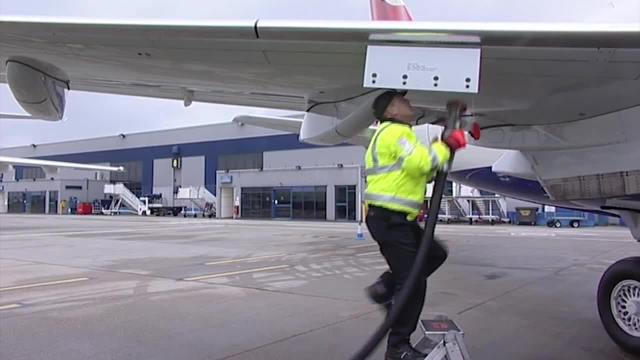 long it would take between the aircraft arriving and then being ready to leave again. We chose to solve the problem using simulation, And the reason we used simulation was because we wanted to make sure that the aircraft would be ready to leave again. We chose to solve. 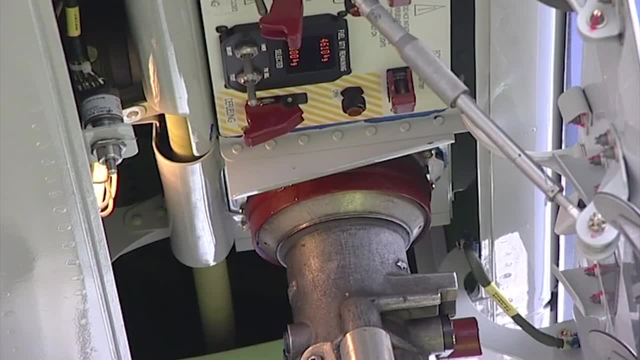 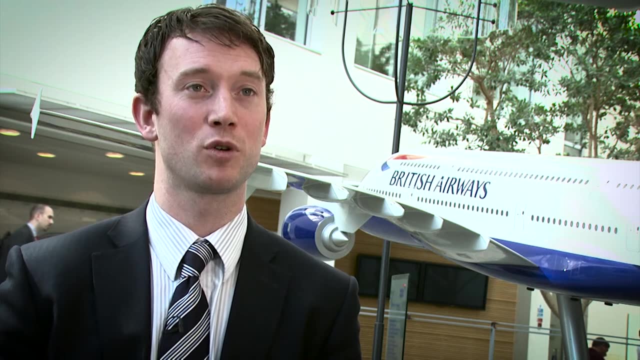 the problem using simulation, and the reason we used simulation was because we wanted to run multiple scenarios in a safe and virtual environment. The best way to do that was by using simulation. We were able to recommend to the business how many staff were required, how many doors we needed to use to board the aircraft to ensure that boarding took no. 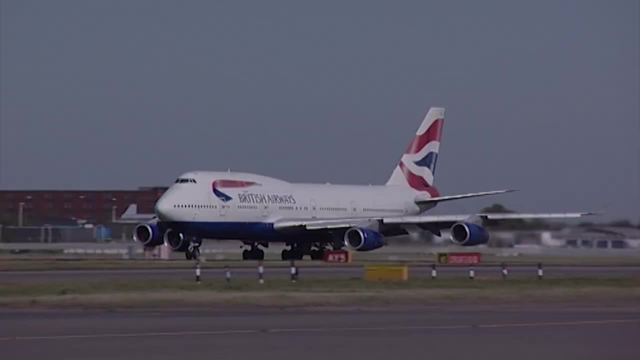 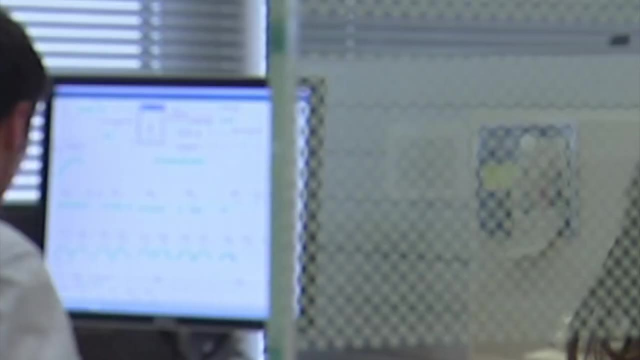 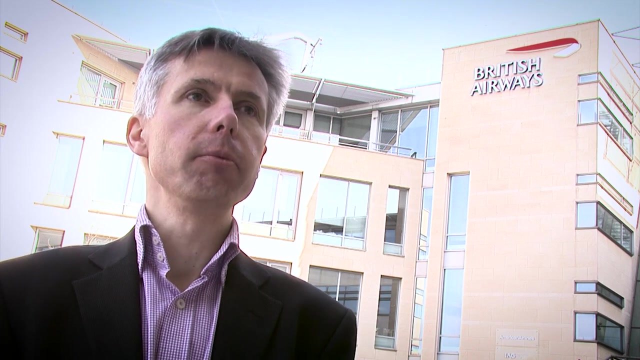 longer than it currently does on the Boeing 747, whilst making sure the customers have the best experience possible. Our customers are really valued here by the company. our thinking and our insights incredibly useful when you're trying to take really difficult business decisions, and also our people often bring that different way of looking at a problem. 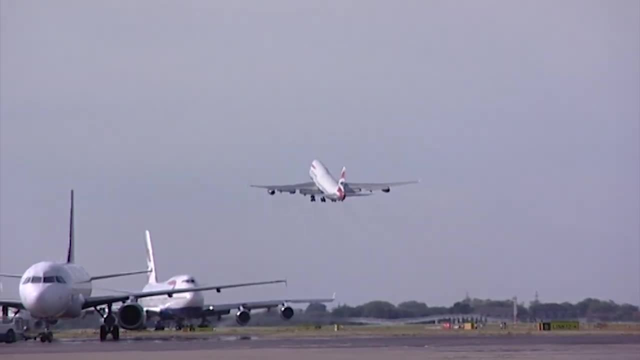 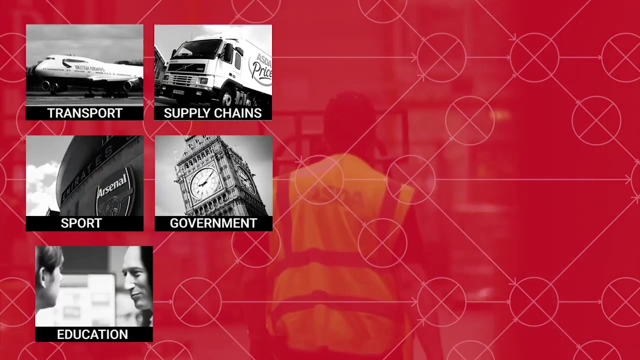 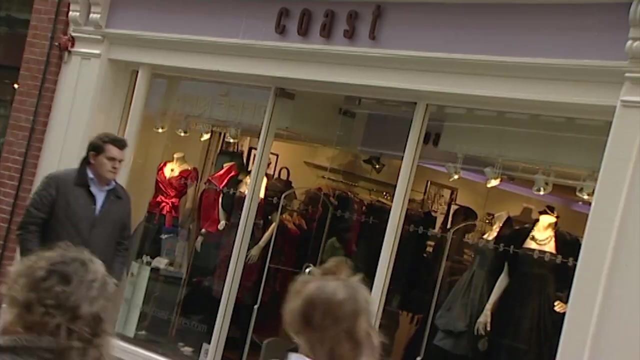 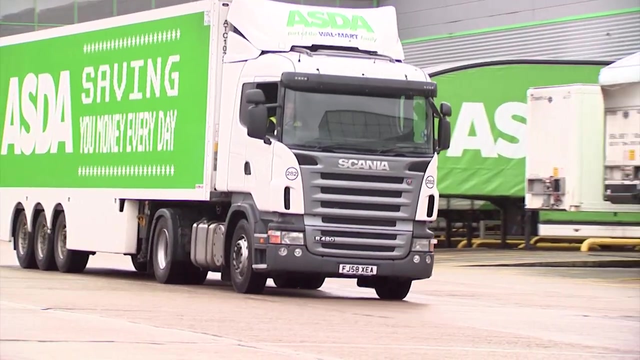 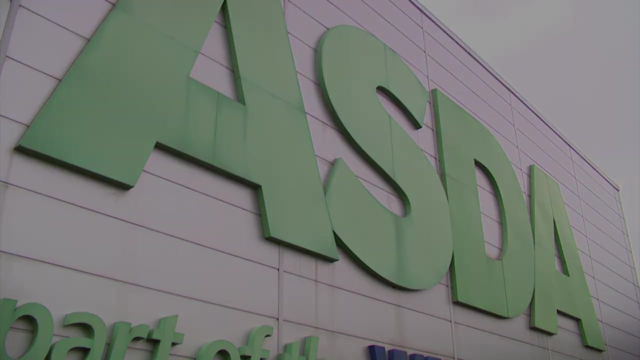 that you, you don't see yourself in today's world. all of us expect the things we want and need to be readily available. that means shelves to be always stocked and deliveries to arrive on time. this is what we term the supply chain of a business. for a major UK retailer like Asda, it's crucial that. 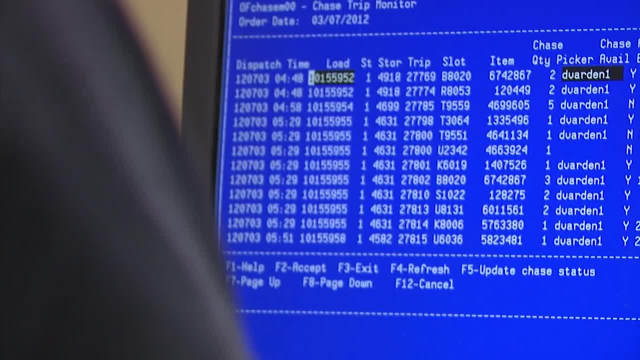 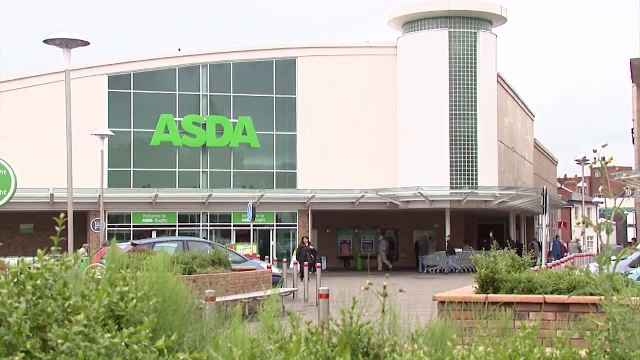 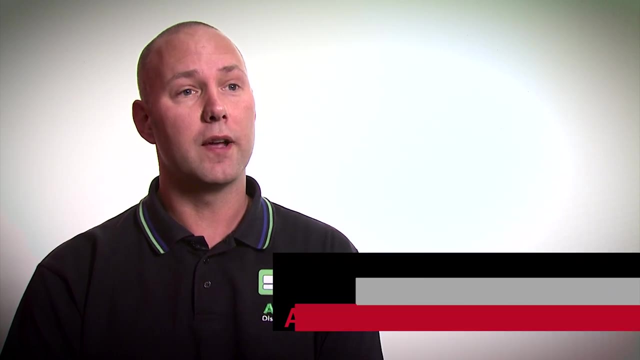 this process runs like clockwork and OR. techniques lie at the very heart of keeping the business running. we service over 500 shops in the UK, serving almost 8 million customers every week of the year. cleaning distribution: we have a huge responsibility to make sure that our customers served on time with 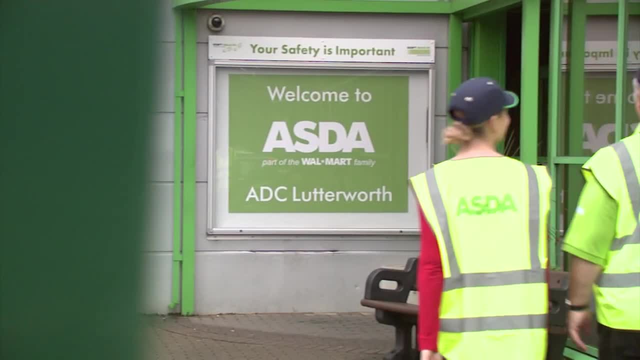 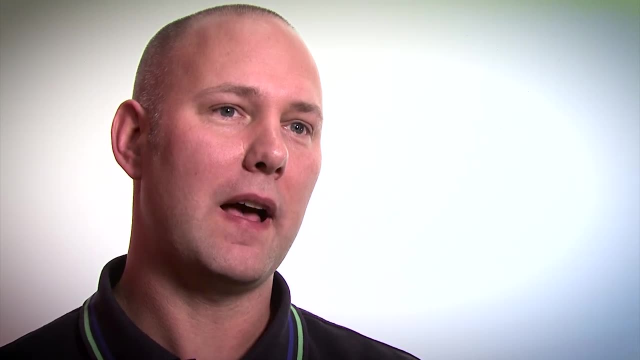 product that's as fresh as possible. we use operational research pretty much every day in our working lives. one of our biggest challenges in the last five years is about how quickly we can get the products from point of manufacturer to point of delivery into our depots, our 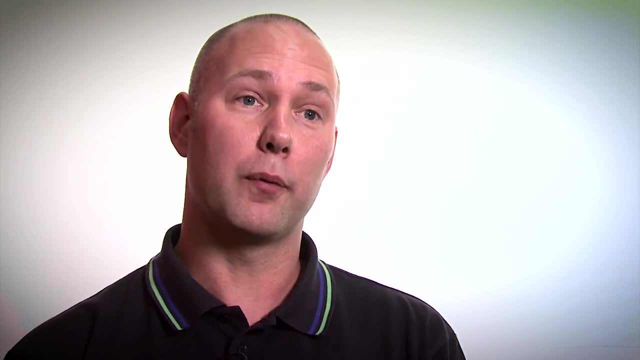 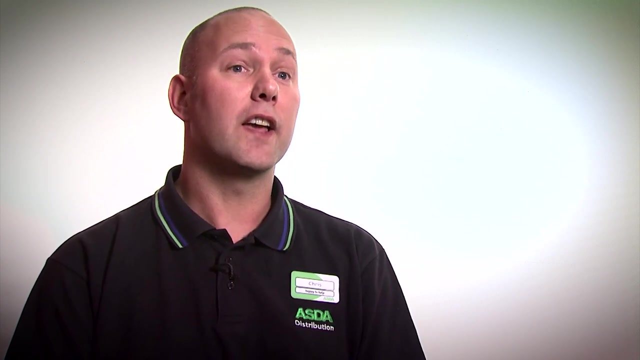 focus on route planning and analysis has made a real big difference to the way that we operate. it means that we take miles off the road. we've reduced the impact on the environment and has helped our cost position. one of our biggest recent initiatives is the utilization of high capacity. 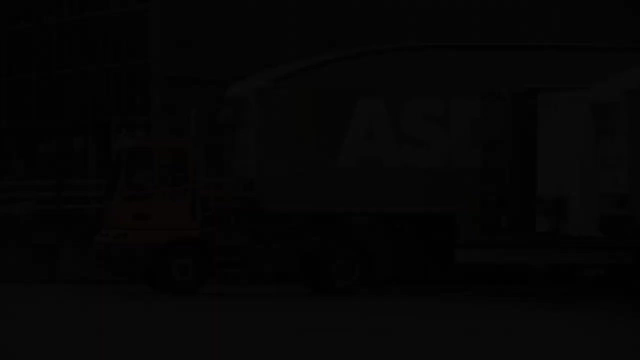 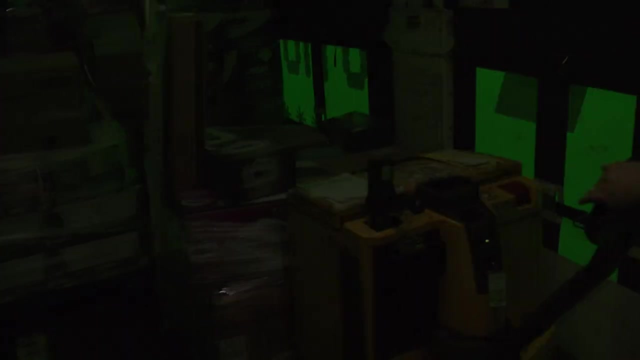 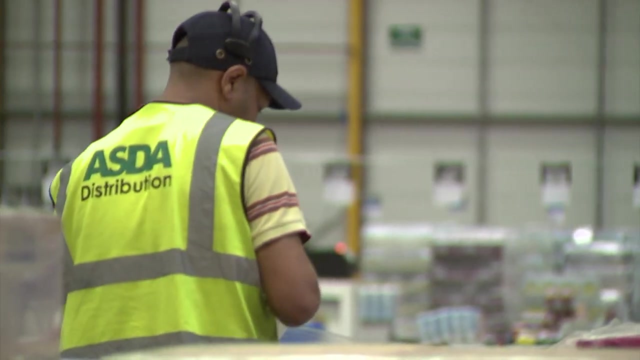 delivery vehicles delivering to our shops. through the analysis that we completed, we were able to prove that by getting almost twice as much product on these vehicles had a substantial cost benefit for us, and it saves us 10 million pounds a year, which can reinvest back into price here at Asda OR. 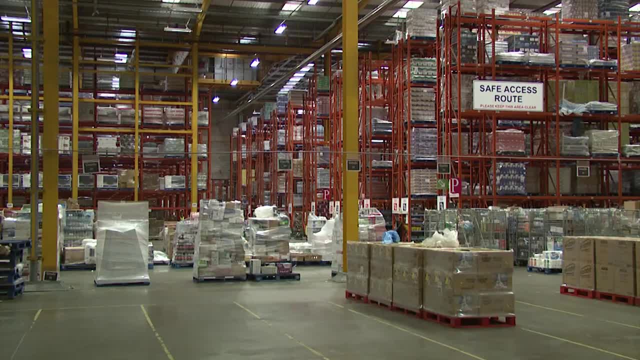 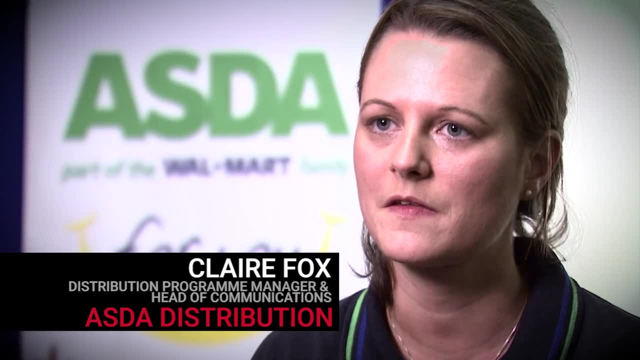 techniques run right through the business, helping to influence big decisions such as where to build a new store or depot. building a new depot is a big investment for Asda and can cost up to 60 million pounds, so it's critical that we build in the right location we do. 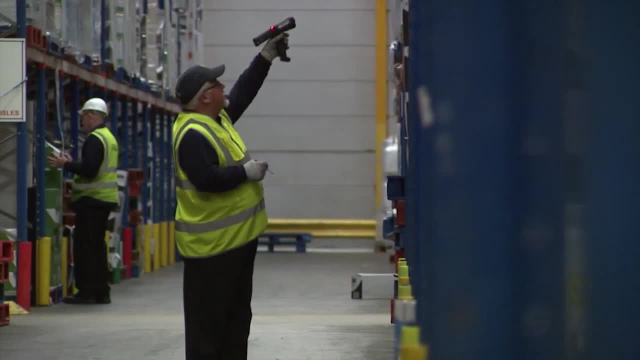 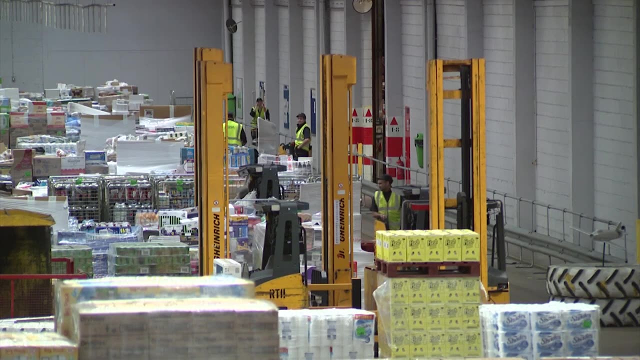 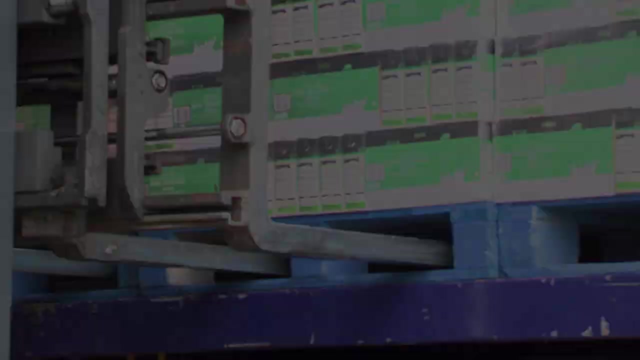 this through a large amount of modeling and analysis tools to help us understand where in the country we will be building new stores, so where that depot needs to be here OR is used to ensure that Asda are constantly improving every process within the depot to get the products out to the stores more quickly. I work in 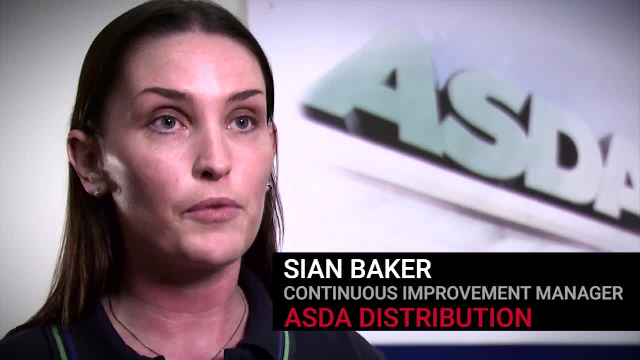 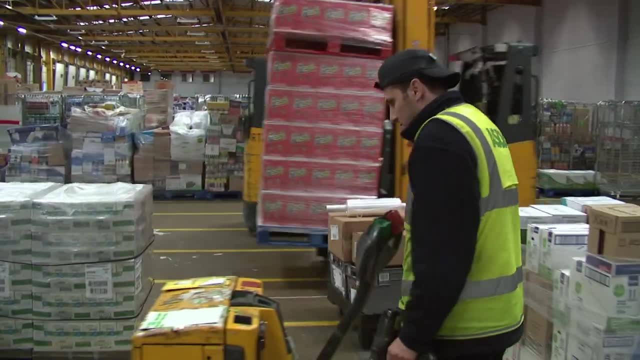 continuous improvement for distribution and we look at our depots and the processes that we complete, how long they take and how we can improve them so that we can make the depot more efficient Every single day that we come to work. it's a new challenge and if we can use 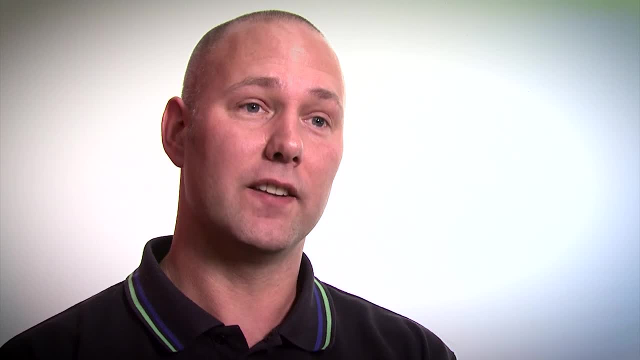 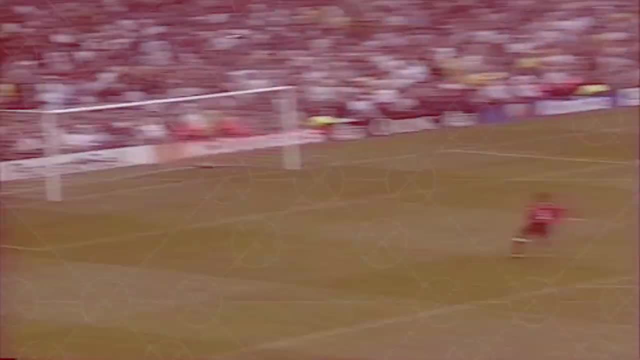 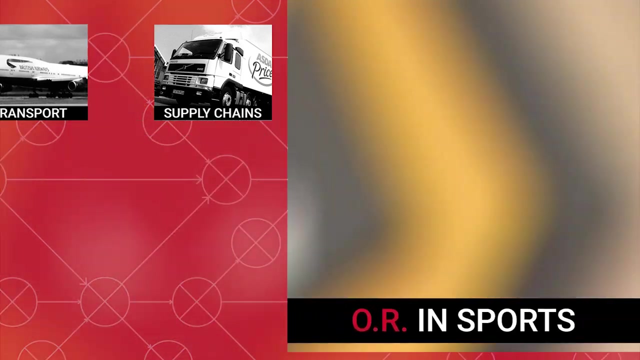 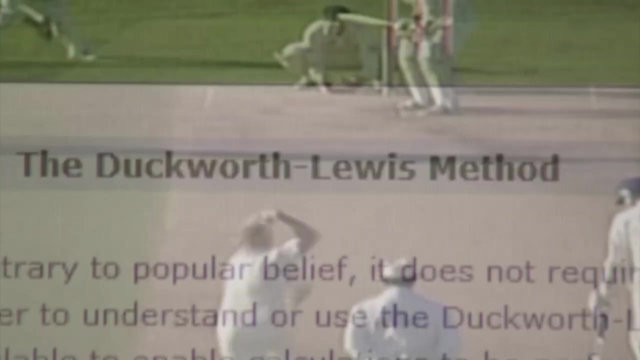 operational research to support that and make it easier and better for our customers, then we've done a great job collectively. The world of sport isn't an obvious place where operational research is at hand. yet many of our much-loved activities rely on OR and whether 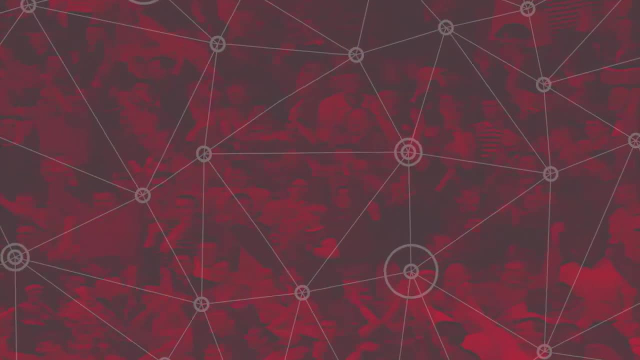 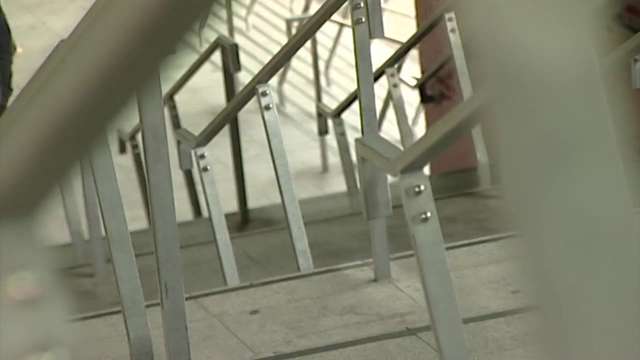 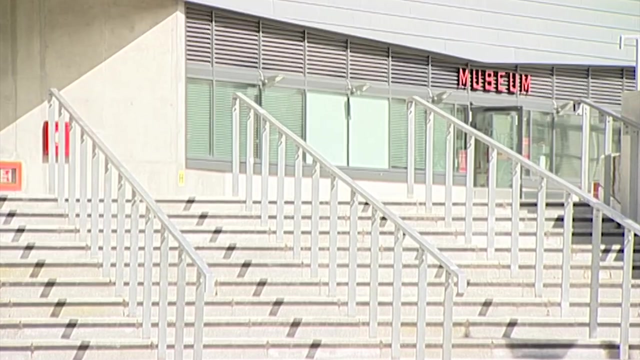 designing a sports stadium or even an Olympic village, OR helps make the spectators experience much more enjoyable. This is the Emirates Stadium in North London, home of Arsenal Football Club. Here, OR had a big part to play in the design and construction of the stadium. 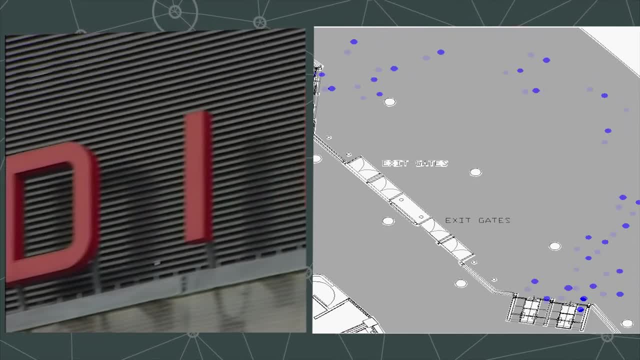 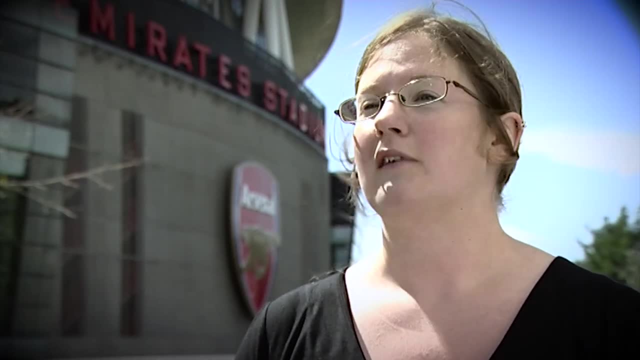 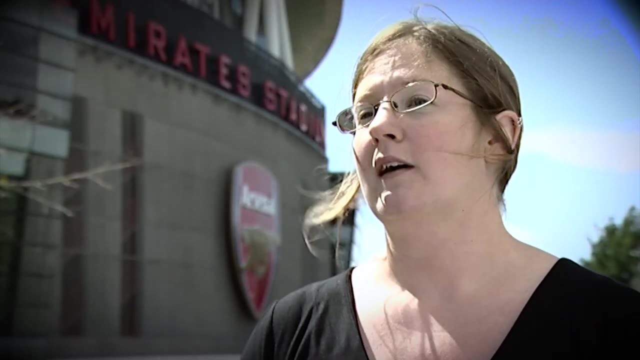 as well as in the efficient running of the site on match day. Just imagine a match day situation when you arrive at the station itself OR starts to feature immediately. You get off the train, people marshal you towards the stadium. That part of the process has already got OR taken into. 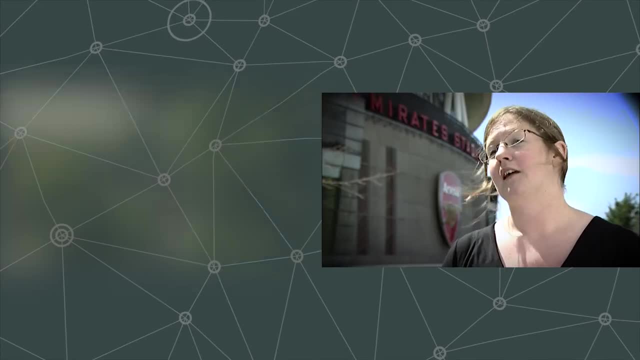 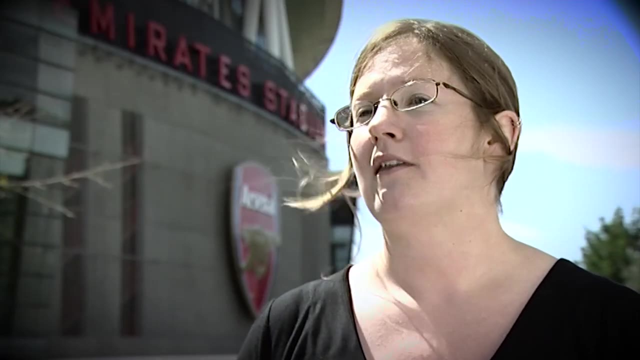 account, trying to find the safest way for you to move. Then, when you reach the stadium itself, the number of turnstiles, for example, will have been determined by an OR technique- and then, as you move around the stadium, the places where the signs are located and the way you move to your 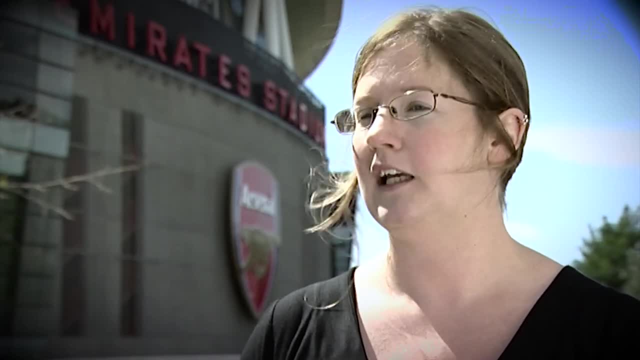 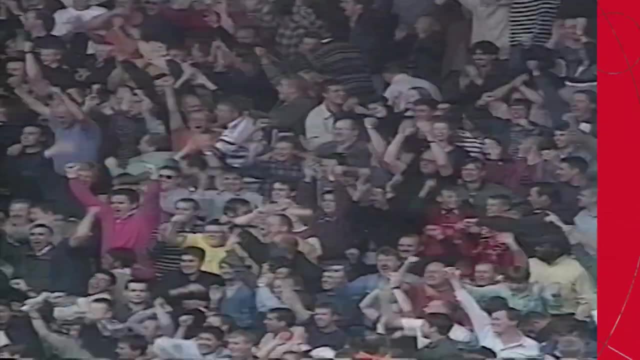 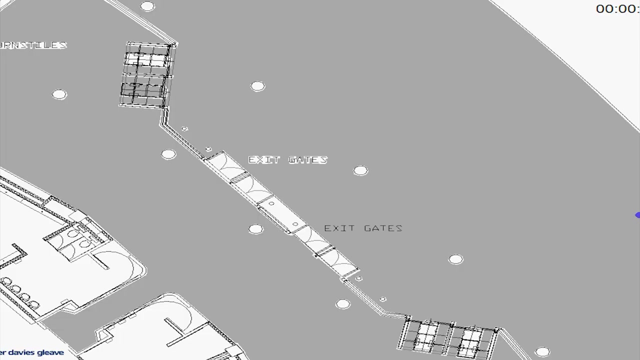 seat will also have been determined by different OR techniques, so it's really important to everything about this stadium. The design of this stadium is obviously magnificent. It's a 60,000 capacity stadium and without a model of people moving in and out, you'd never. 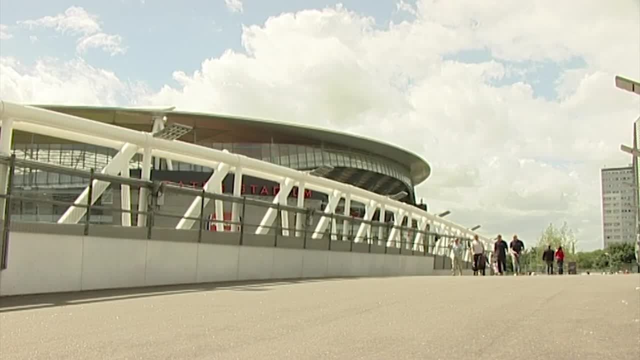 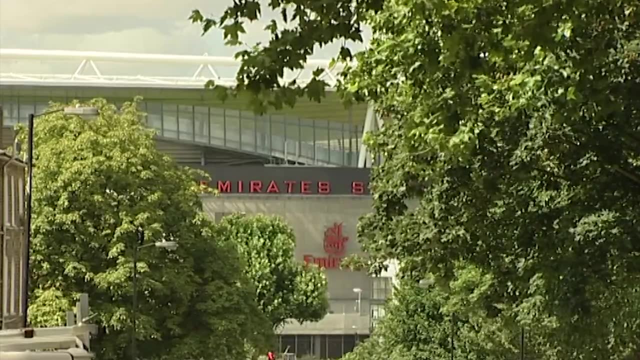 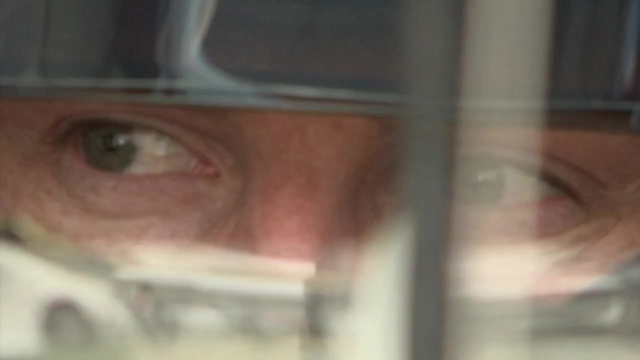 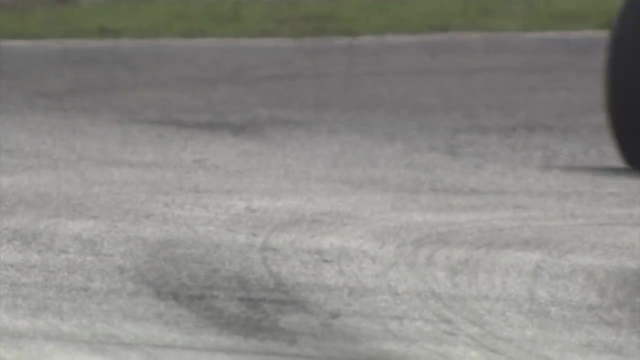 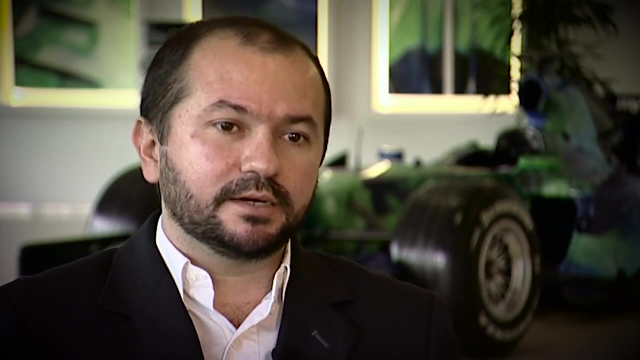 know whether, during a match situation, if there was a fire, for example, if those people could be evacuated safely within the eight minute guidelines. The explosive world of Formula One: High speeds, Multimillion pound racing technology. During Formula One, we require more and more people to return to our stadium. 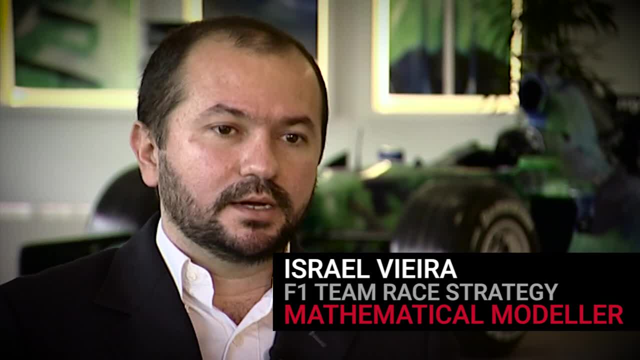 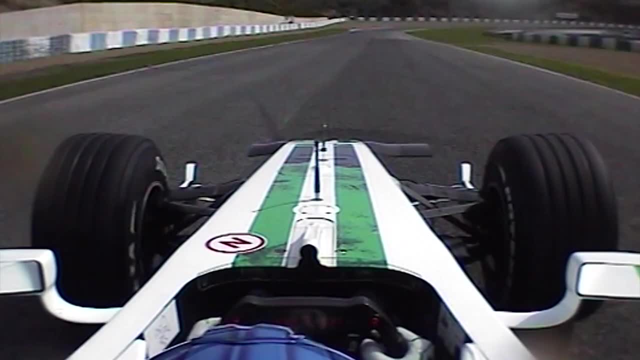 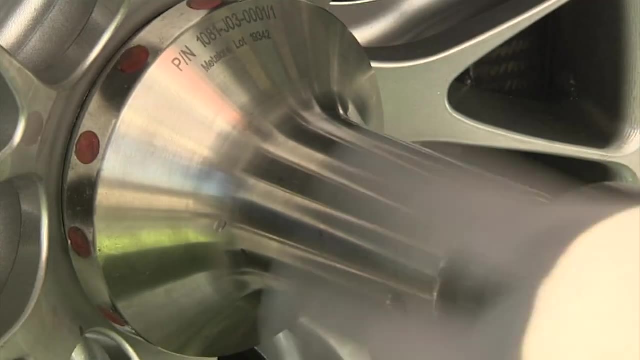 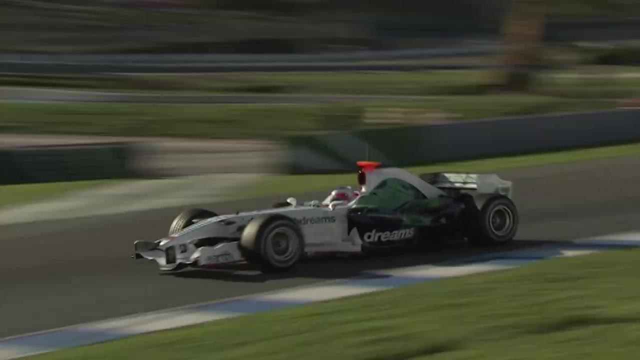 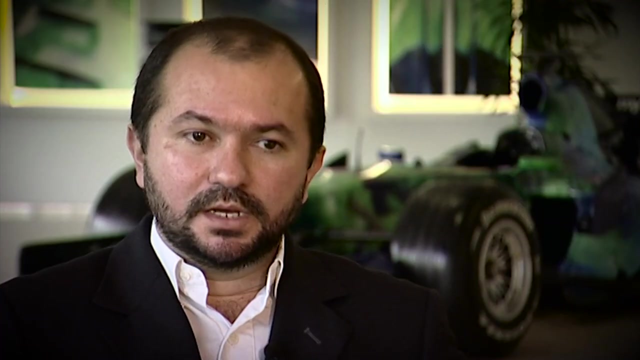 more expert on risk analysis and game theory and simulation, Formula One, where split-second decisions are the difference between success and failure, And often these decisions are a matter of mathematics resting in the hands of some of the world's finest operational researchers. I think the first thing that people see the direct application of OA is on the fine. 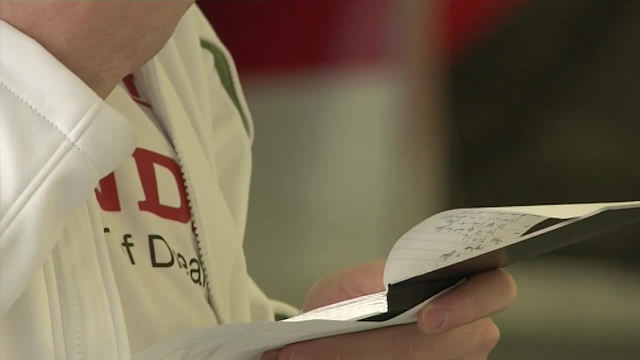 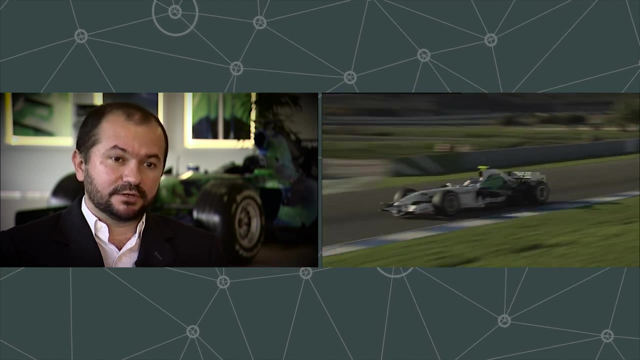 the race strategy, the initial fuel load, Estimating competitors' fuel load and where they're going to stop and when we're going to hit traffic during the race. when is a good lap to come out of the pit stops and tire degradation? 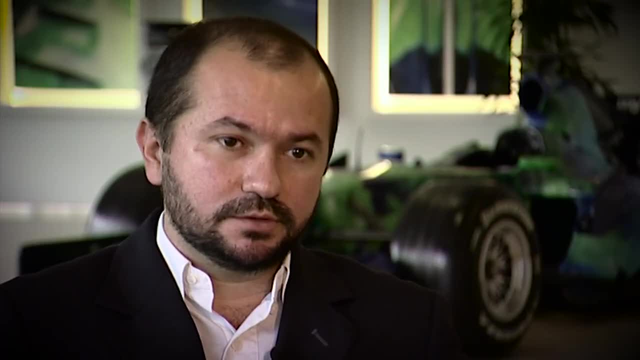 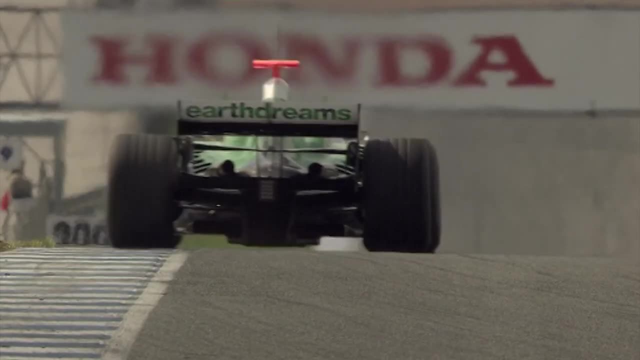 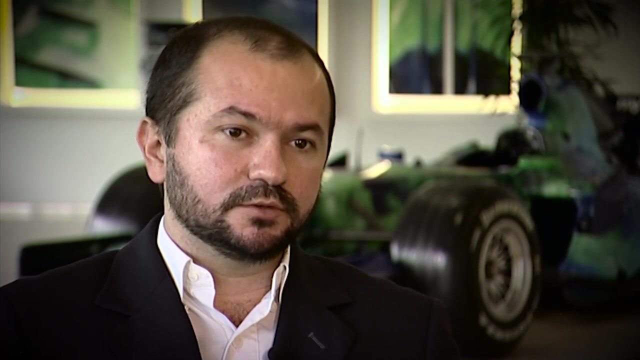 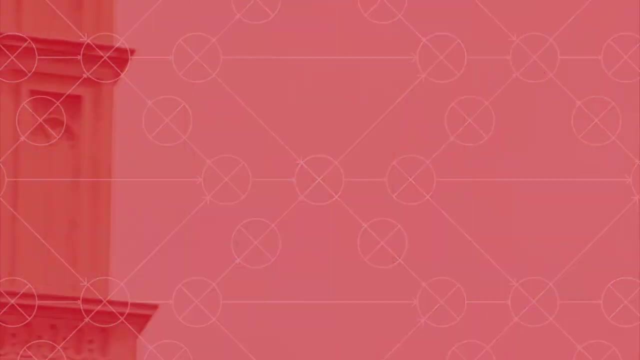 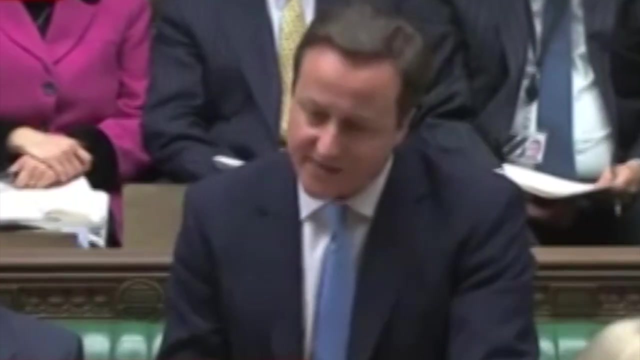 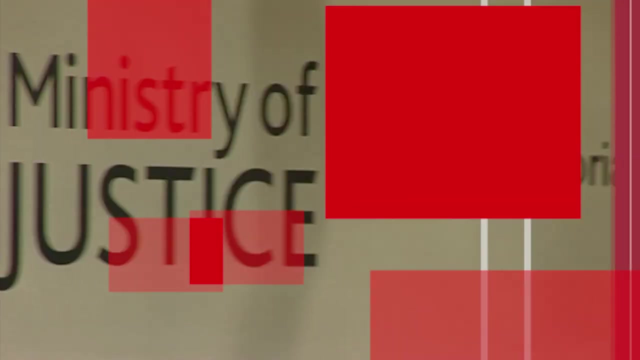 This is all estimation that we need to do as the race develops. I strongly believe that OA has a great role to play in Formula One for the future. Central government is the biggest business in Britain And in government OA gets involved in just about everything that affects our day-to-day. 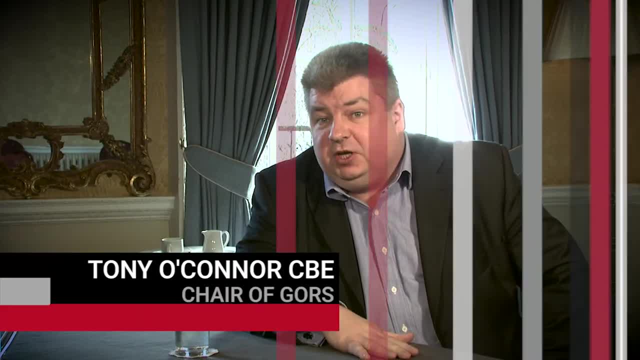 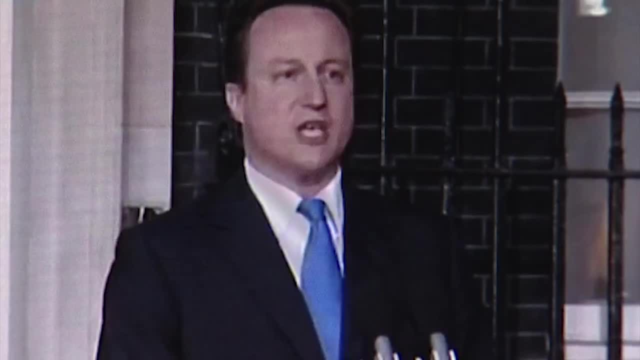 lives. Operational research plays a crucial role in improving the quality of decision making right the way through the system, from senior decision makers in departments right the way up to the Prime Minister. If you've ever interacted with schools, obviously you have, or with hospitals, or with the transport. system, you'll have had some benefit from the role OA has played in improving the way that those services are delivered. Or, essentially, looking at OA'sこと as well as the cost, I've always wondered how it is our responsibility to make. 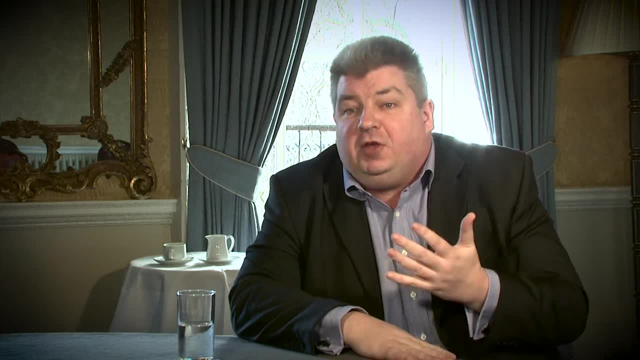 organisations better and to get it to keep us out of the way, But, I think, at the same time, coming across potential audiences in the future as well. we're delivering the things that we all live and breathe and interact with on a daily basis. 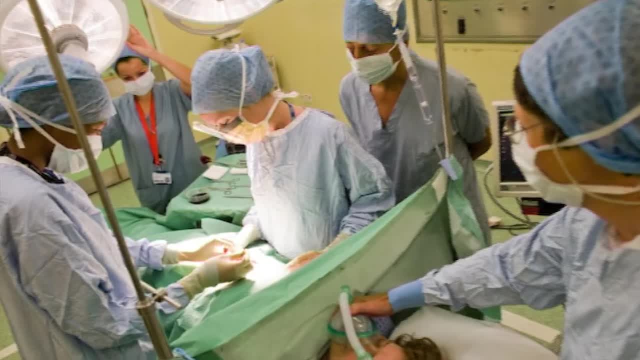 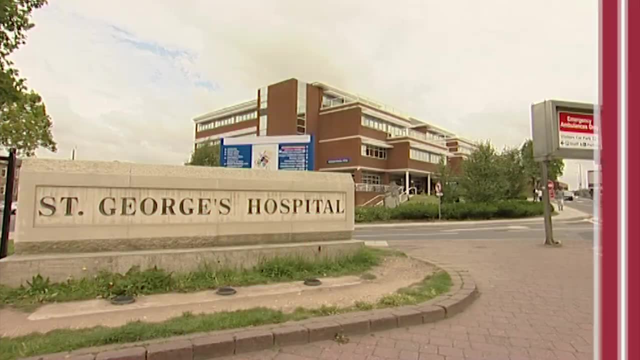 This is St George's Hospital in London. Here, using OR techniques can literally be the difference between life and death. One of the really big things that hospitals have to think about is how long patients stay, and so, therefore, how many beds and how many wards and how many doctors you. have to look after them. It's really important for us to be able to get, as far as we can, the right capacity for the patients who are going to come through the door so that we can give them the treatment that they need when they need it- Patients when they're referred by their GP either. 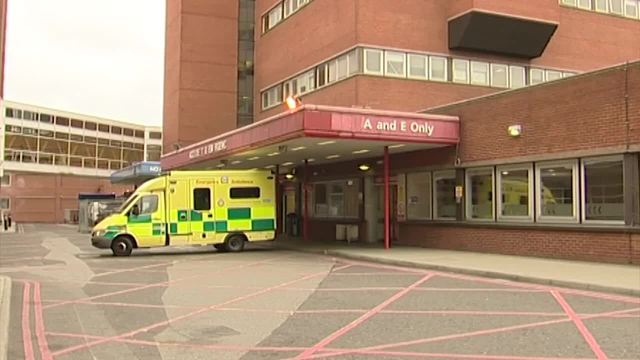 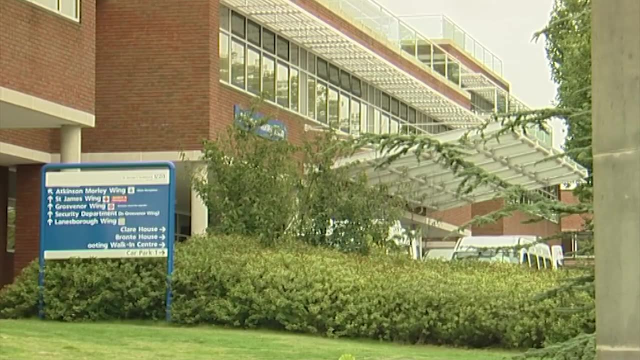 into A&E or into outpatients enter a series of queues, and one of the things that we really have to do- and we've been working very hard on- is getting those queues as short as we can and making sure that we don't have bottlenecks in the hospital. 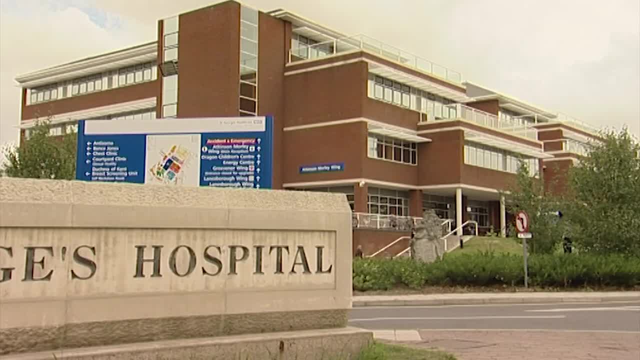 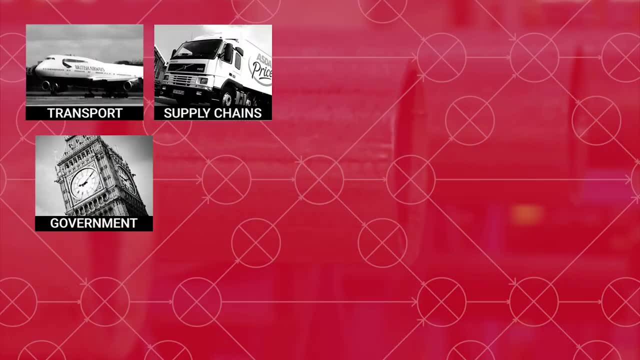 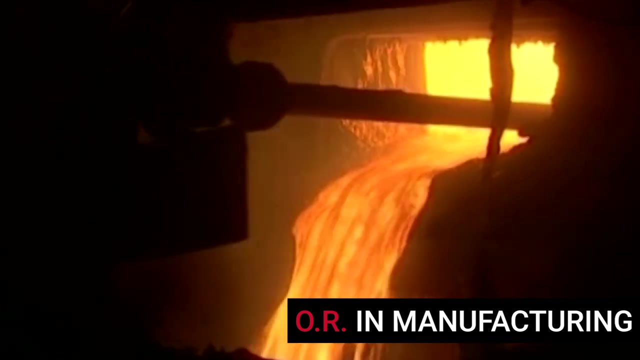 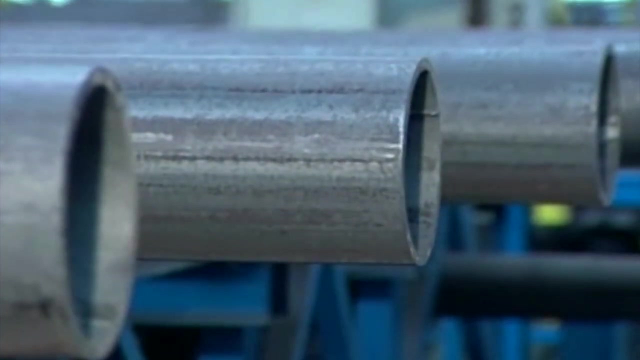 In our system, and so, therefore, we need queuing theory and operational research techniques to help us make sure that we can get that right. Operational research is often at the heart of what makes a business run efficiently. Here, everything must be planned and timed precisely to avoid bottlenecks. 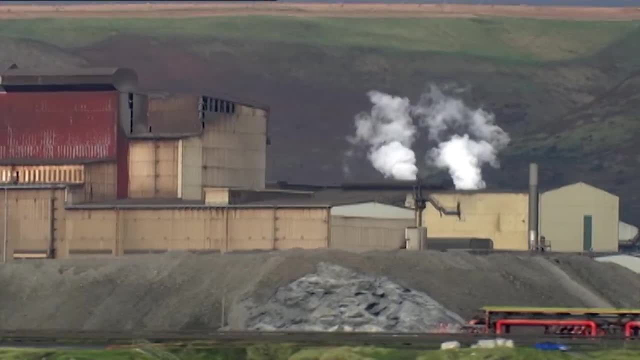 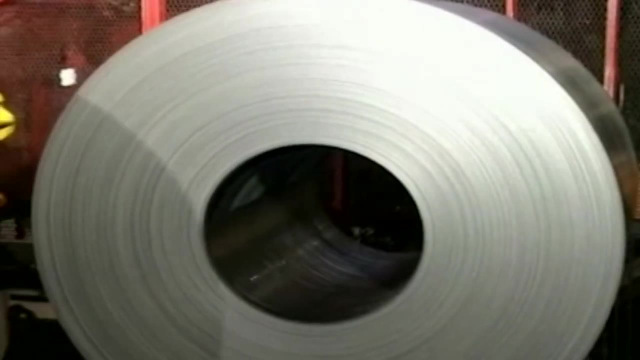 Tata Steel manufactures steel products, and operational research is a key part of the business. Tata Steel manufactures steel products, and operational research is a key part of the business Here. operational research techniques are key to improving productivity and reducing costs. What we produce here are big steel coils that we sell on to. 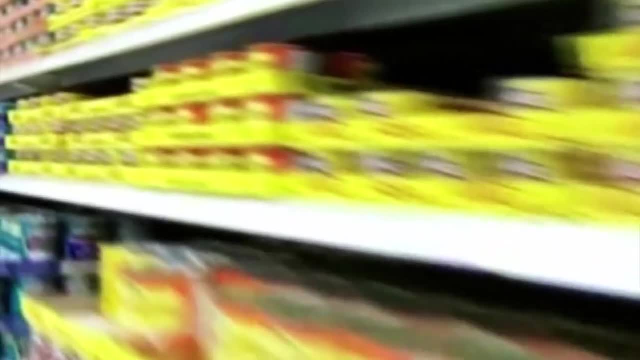 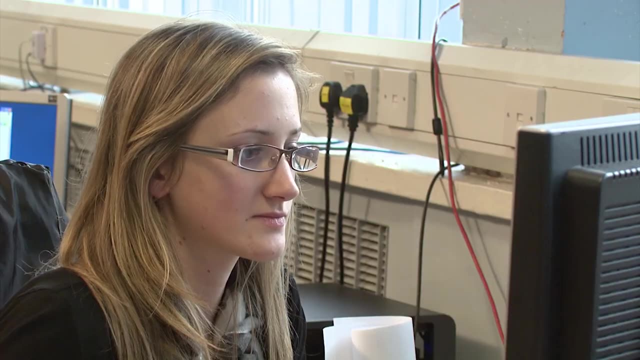 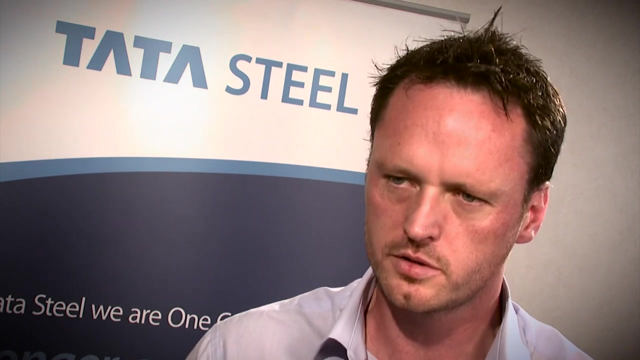 various companies that produce everyday objects such as tin cans, office furniture, cars and fridges. The OR team currently consists of 12 members. We provide an in-house service where we incorporate ourselves into various project teams for all the departments. We use lots of software within the department where 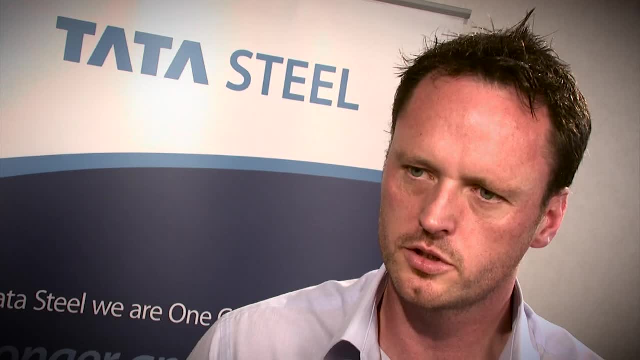 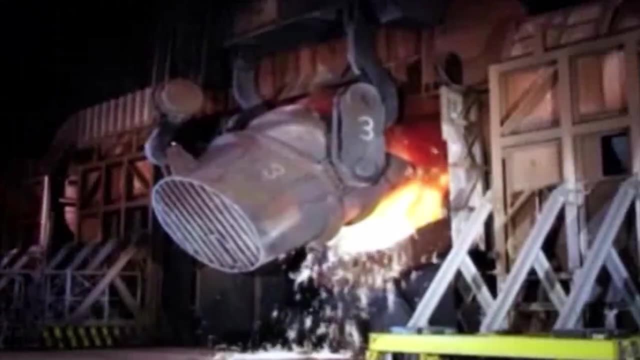 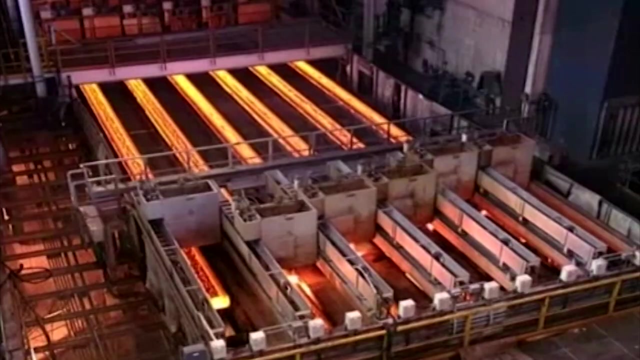 we can build real-world processes on a computer screen and visually show these to the project managers, the process specialists, and they can play out various scenarios without having to work them out on real-world processes. This, in turn, can save a lot of money and is a lot safer in the long run. 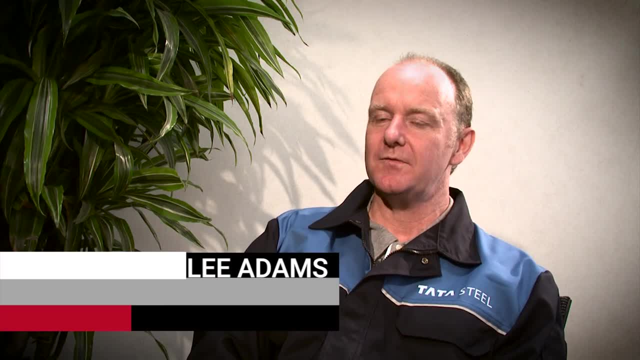 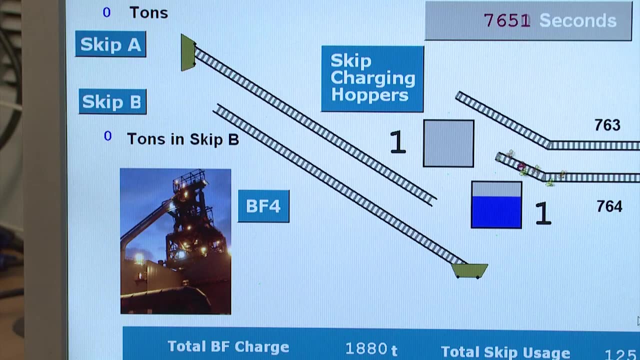 Here on the plant we've had a throughput of up to 4.4 million tons of steel and we're looking to take that up to 5.3 million tons. So we've got a project to look at the infrastructure to see if it can handle the extra 20% throughput. 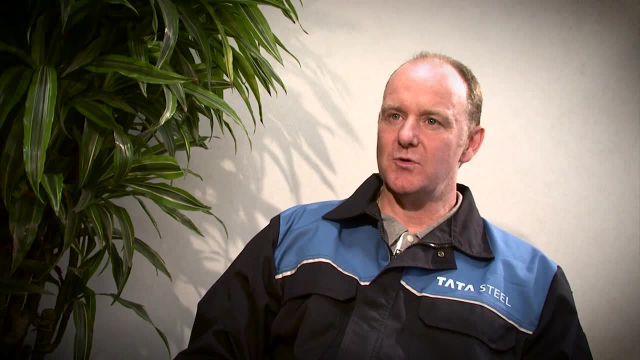 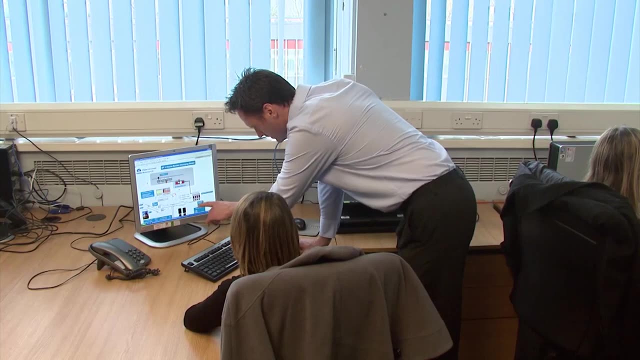 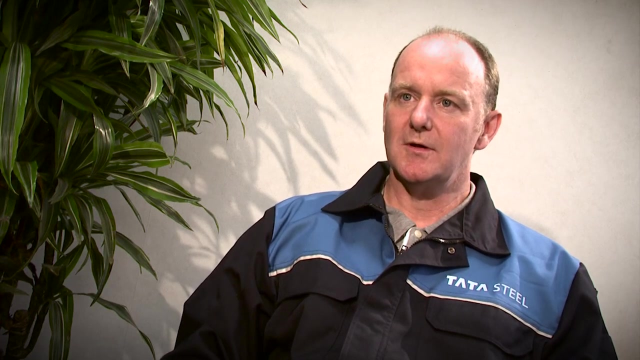 The benefits of producing 5.3 million tons as opposed to 4.4 will mean that our cost per tonne will come down as an organisation. The reason why we got the OR team involved is because when you're looking at your own process and you're so close to it, I think you make a lot of. 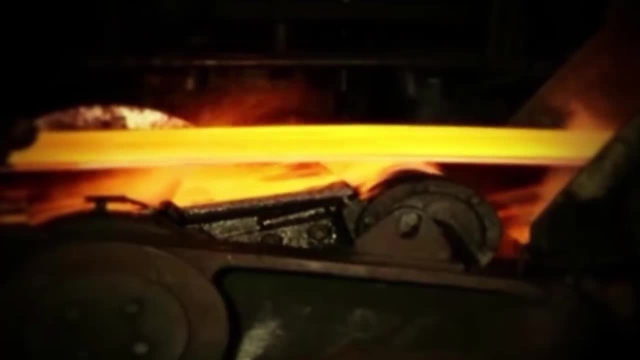 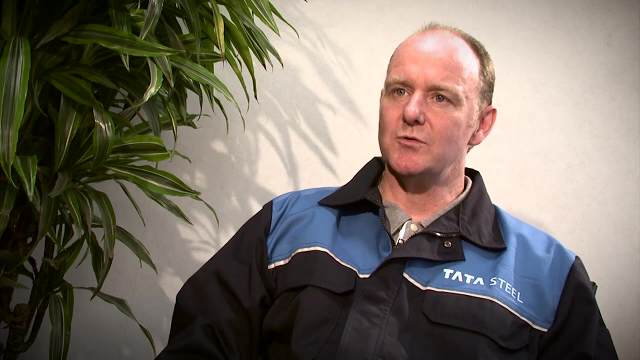 assumptions and the model will take those assumptions away. They started coming to our meetings first of all, but then we got into the nitty-gritty process, Actually going out on plant and getting them as close to the process as we could so they could see for themselves. 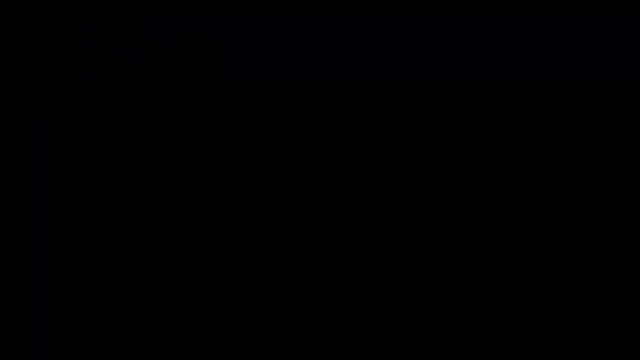 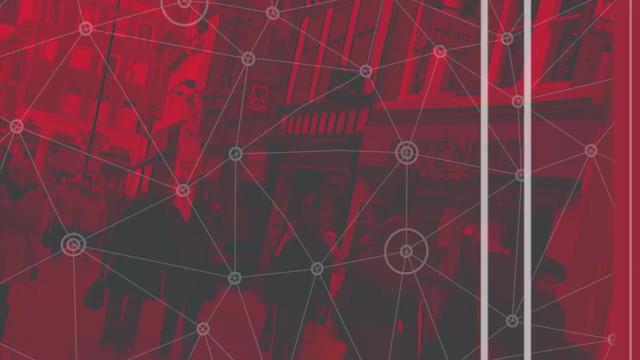 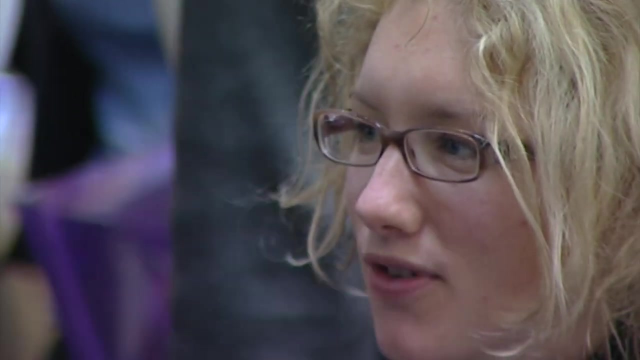 As you think about what the future may hold for you. if you want to consider taking up a career in operational research, take a look at the interesting university degrees out there that are the best route into what we call OR the science of better. 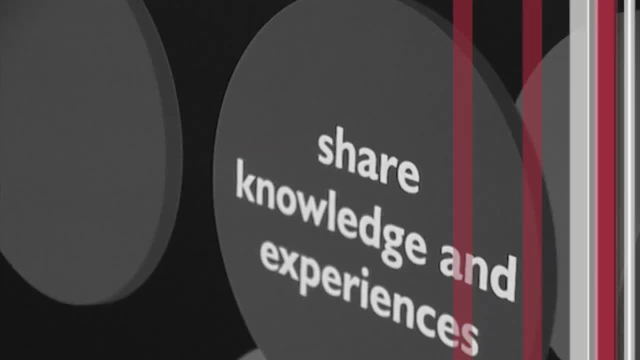 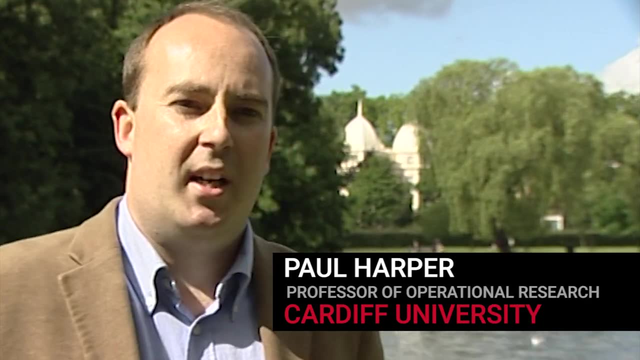 Offering you a truly inspirational challenge that will test even the most inquisitive of minds. There are many different academic paths into operational research. although most people tend to have degrees with mathematics, statistics, computer science or management content, Pupils will learn a number of OR techniques, such as: 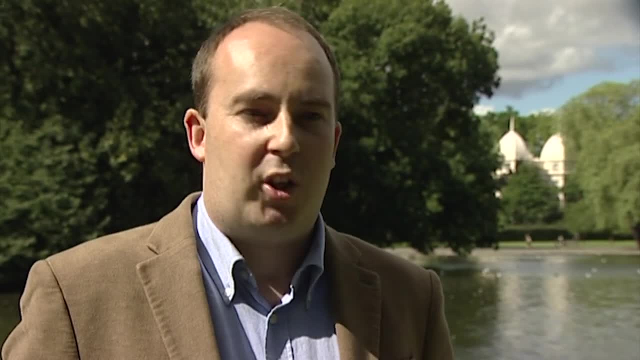 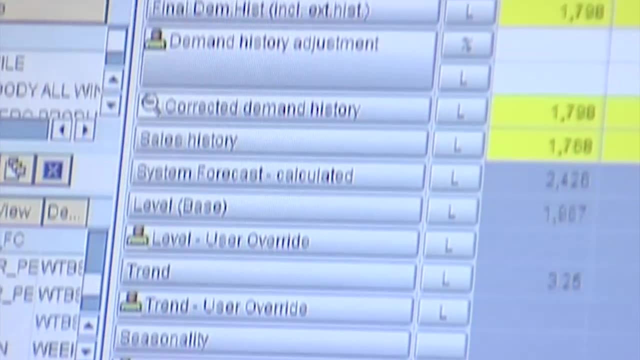 computer simulation, optimisation, queuing theory, inventory control, problem structuring methods, to name just a few. You also get a good balance between a theoretical work and an appreciation of the application of these techniques, and that will involve case studies, project work, which might involve a lot of work.